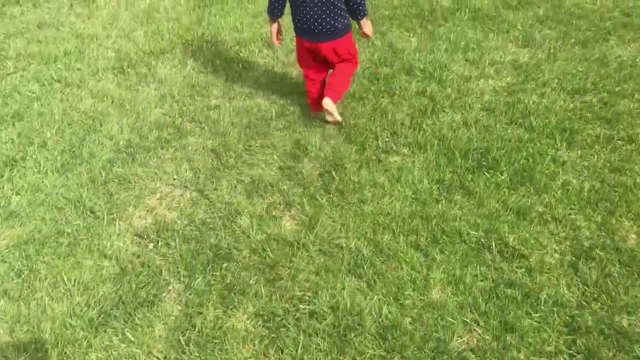 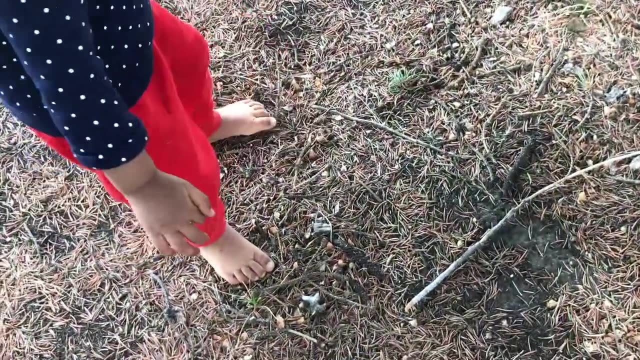 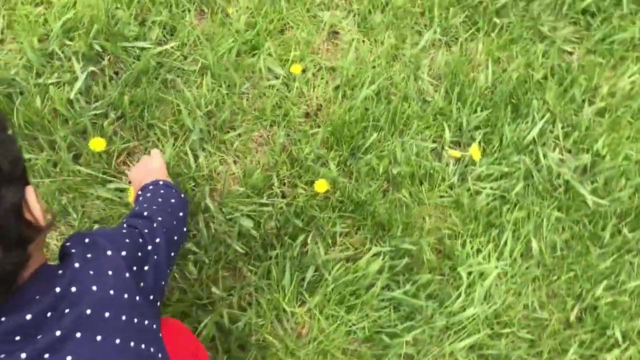 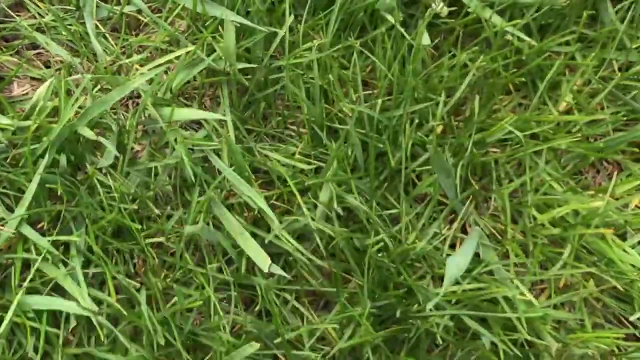 After that I let my baby graze in the grass and we did some relaxing activities for them. Many of them had a reaction to the sensations and the sensual sensations. This was just a beginning for them to understand the difference between the sensation and the perception. 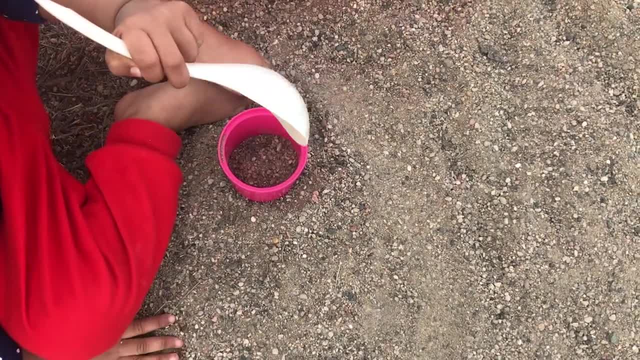 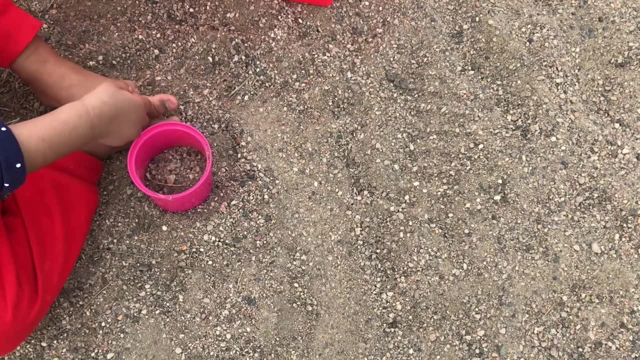 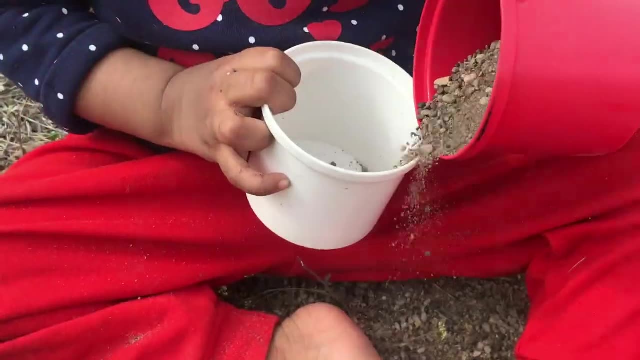 So we all know that sensation is the process by which we just sense our surrounding environment through using our sensory organs such as touch, taste, sight, sound and smell. on the other hand, perception is the second stage of the sensation. while doing perception, we interpret the information we receive through sensation. so, by doing 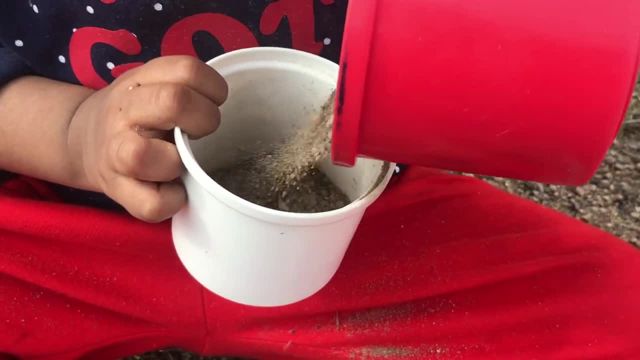 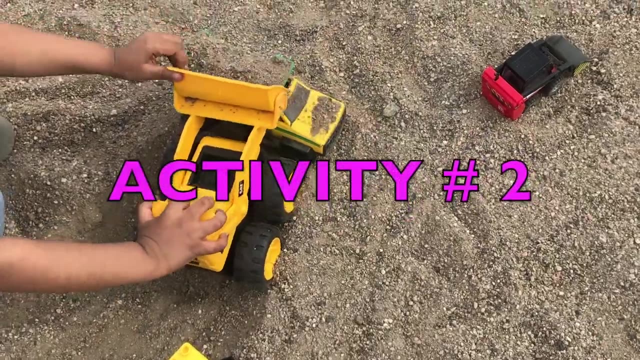 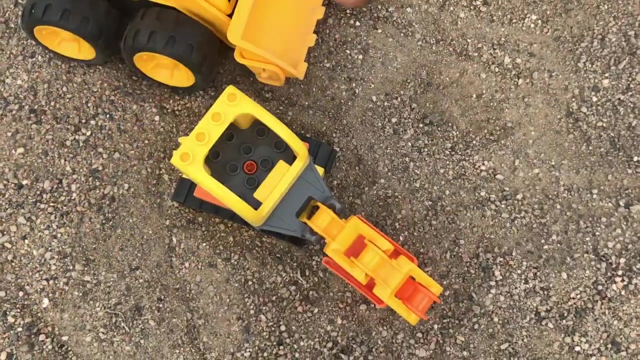 these type of activities we we try to motivate our brain to interpret different perceptions and come to a conclusion. next activity was who all can see was a sand play and it was a very fun and engaging activity for my kids. my son especially enjoyed his construction play in a sand. he enjoyed digging, pushing. 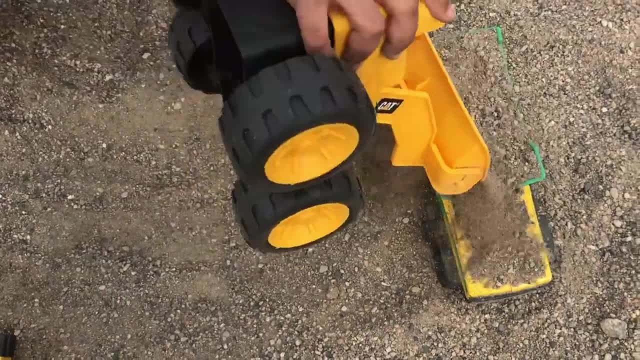 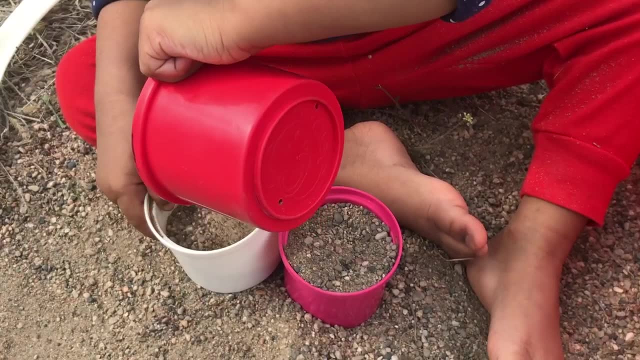 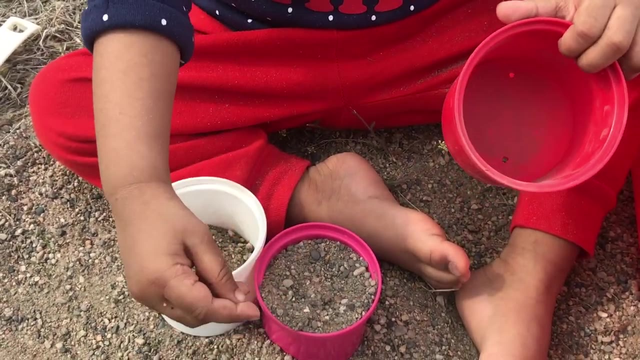 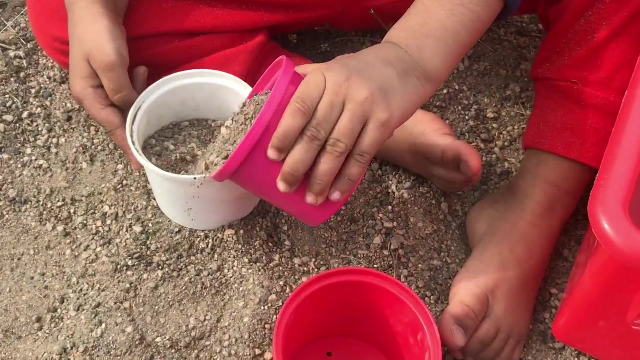 and dumping sand in his construction toys. at that time, weather was very windy and it was getting difficult for us to do our sand play, but despite that, we were able to sense the flow of wind on our body and then observe how wind can do its magic, like blowing the sand away. 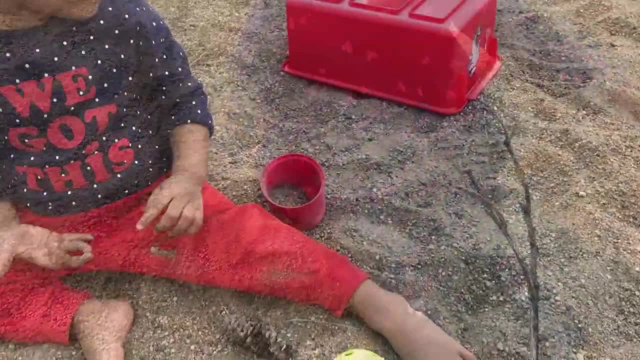 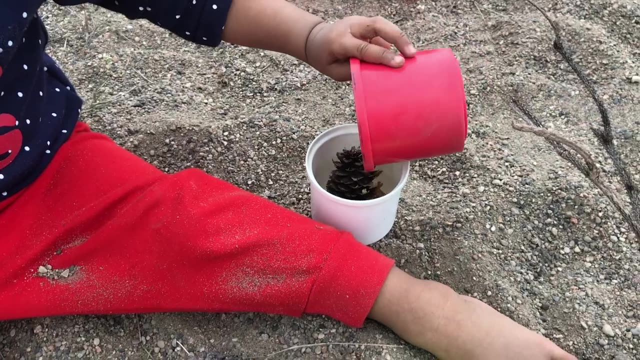 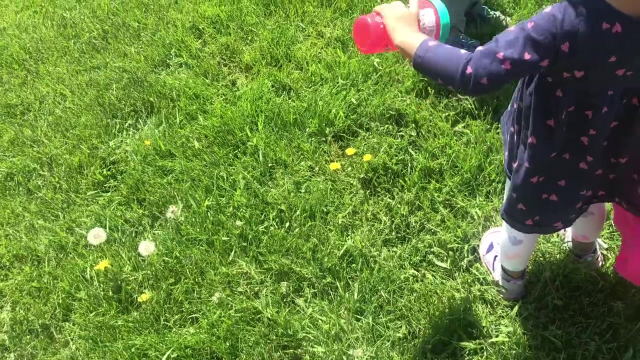 there is a plethora of research supporting that spending time in nature can be many positive benefits to humans: physical health, emotional health and for their overall well-being. so doing these types of activities, we empower our kids for having a very healthy and balanced life. next activity was simply going for a nature walk. during our walk, we gave 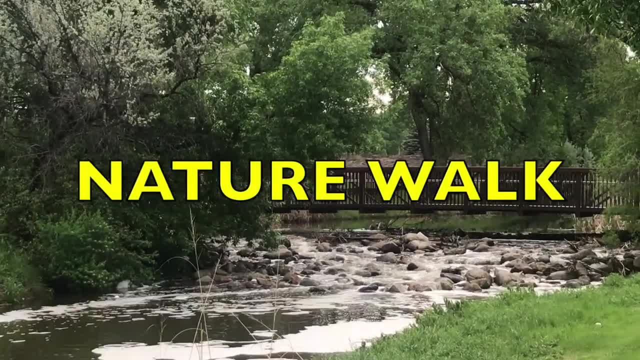 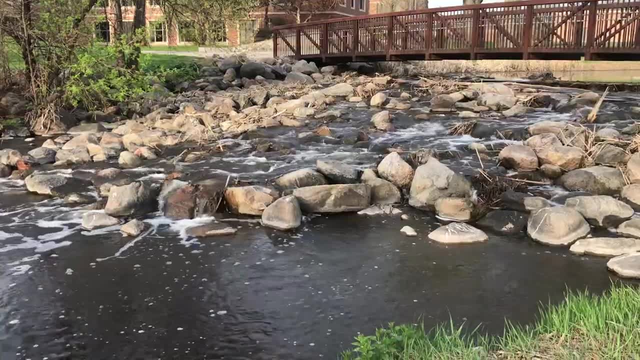 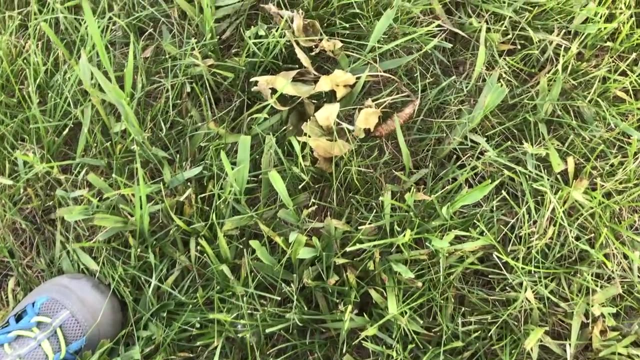 focus on spending time in nature and viewing nature scenery. we watch movements of trees and leaves in a strong wind and paid attention to water flow in the stream walk. interestingly, we were able to watch and spot a lot of birds and small creatures. kids were especially happy when they saw small creatures like cocoon.